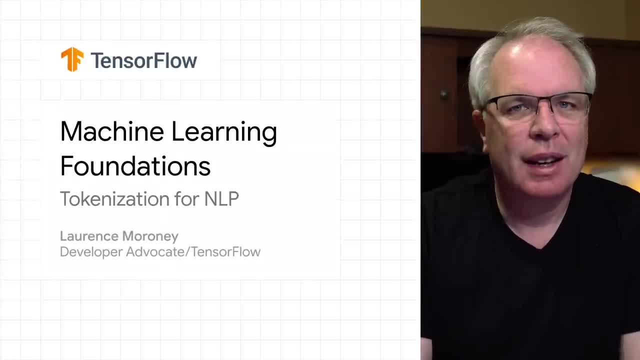 Hi and welcome to episode eight of Machine Learning Foundations. I'm Lawrence Moroney from the Google AI team and I'm here to be your guide through the basics of machine learning. Up to now, you've learned how machine learning works and explored examples in 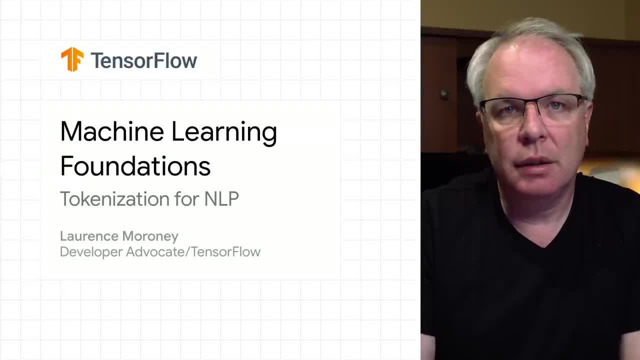 computer vision by doing image classification, including understanding concepts such as convolutional neural networks for feature identification and image augmentation, to avoid overfitting, making your networks that little bit smarter. We're now going to switch gears and we'll take a look at natural language processing. In this video, we'll take a look at 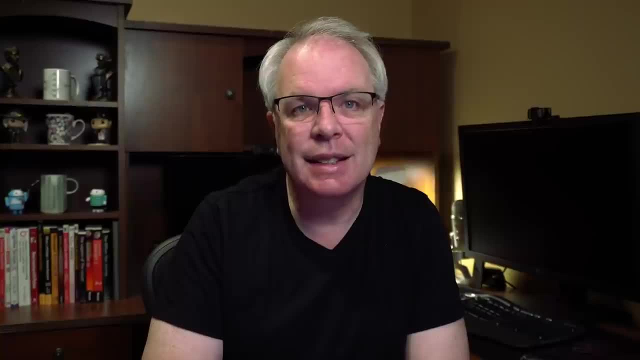 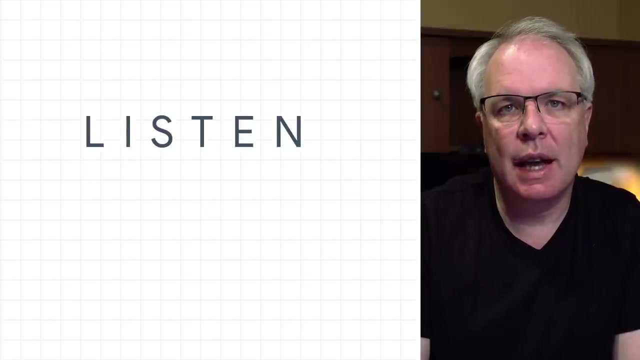 how a computer can represent language, and that's words and sentences, in a numeric format that can then later be used to train neural networks. This process is called tokenization. So let's get started. Consider this word. It's the English word listen and it consists of six letters. 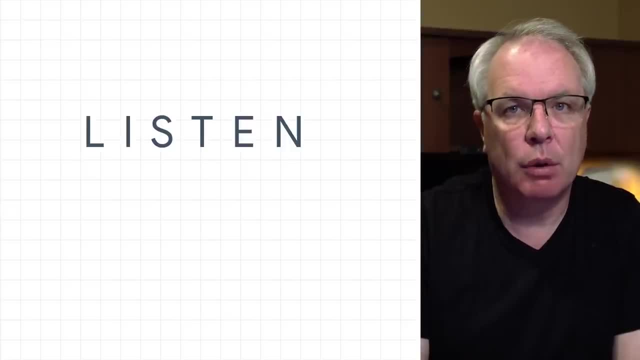 We're used to reading it based on the sounds and putting those sounds together to form a word. But how can a computer understand this word? Well, one way, as computers deal better with numbers than they do with letters, is to assign a number to each letter. A common coding format is called ASCII. 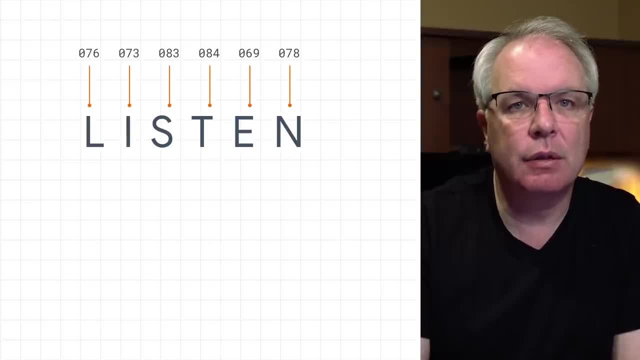 where common letters and symbols are encoded into the values from 0 to 255.. It's useful in that only one byte is needed to store the value for a letter, but it has been superseded by later encodings in order to give access to characters and. 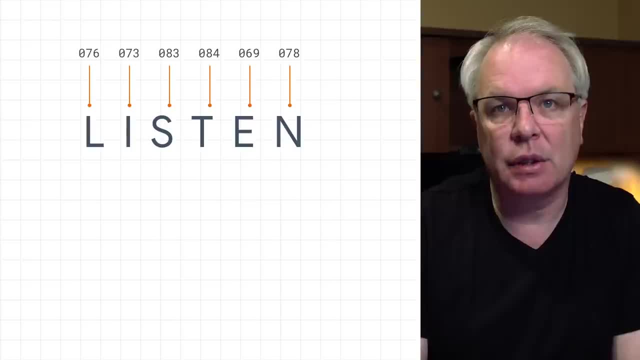 letters beyond 255, in particular international characters. But for the purposes of illustration we can stick with ASCII, where, for example, the letter L is 76,, I is 73, and so on. So we now have the word listen encoded into six bytes, one for each letter. 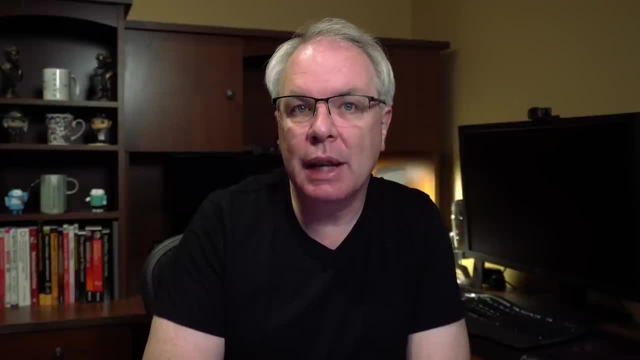 Now, this is a perfectly valid encoding and often when you use neural networks you'll see character encoding or sub-word encoding and stuff like that. They lead to things being a little bit more complicated, and in these tutorials I'm going to do word-based encoding and not the letter-based that we just saw. Now why would I do that? 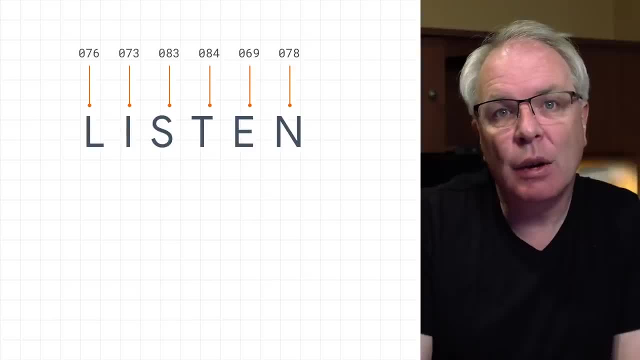 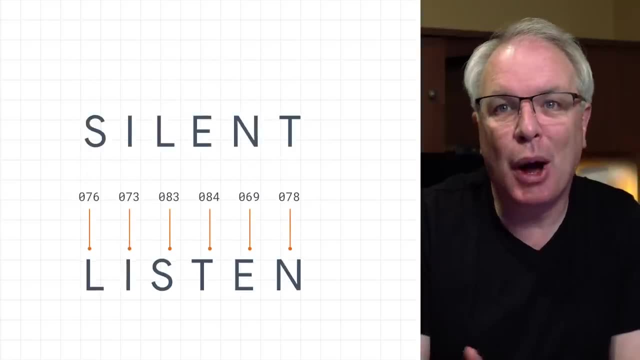 One reason is that if we're taking a word as a set of numbers, unless we take the sequence of those numbers into account, we can have two words, sometimes with opposite-ish meanings like this, and they can have the same letters. Thus, if we want to use character-based encoding, 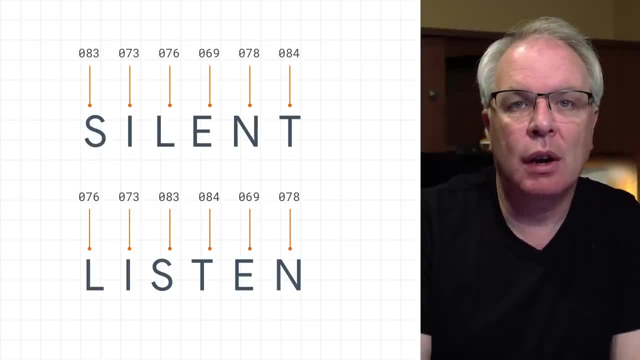 a computer can't tell the difference between these two words unless we have a sequence model, and that's a little bit more complicated than we need to look into right now. So let's consider a different encoding, and that's a word-based encoding. 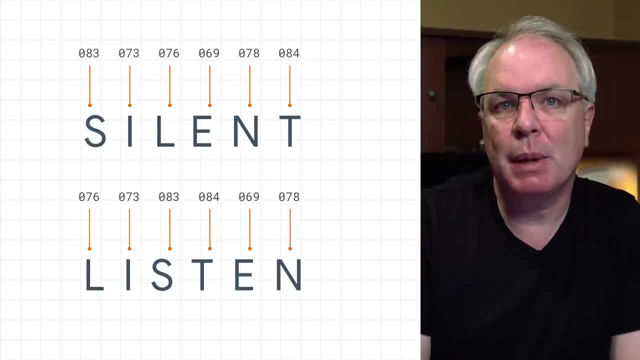 That way, each of these words can be represented by a single number, and each number will be different. There's also a nice hidden advantage to this, which we'll see in a moment. So consider this sentence: I love my dog. It's a pretty straightforward one. 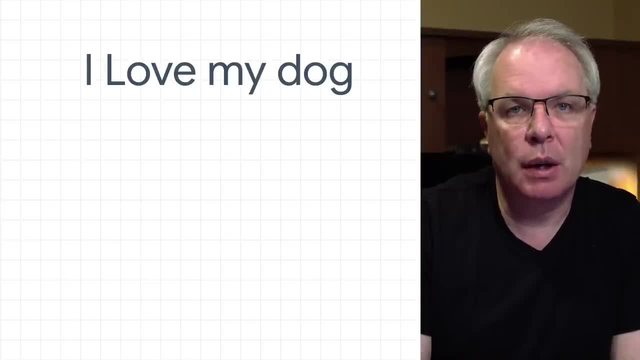 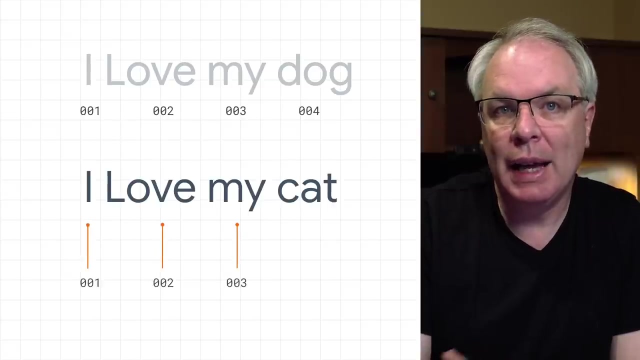 If I encode based on words, I can come up with an arbitrary encoding. Say the word I is number one and then love my dog, become two, three and four respectively. Now if I were to encode another sentence, for example I love my cat, the words I love my already have numbers. 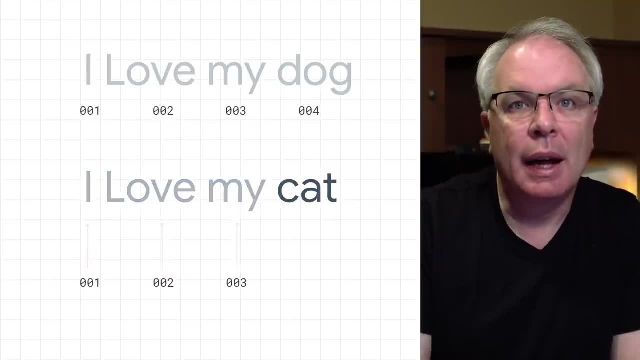 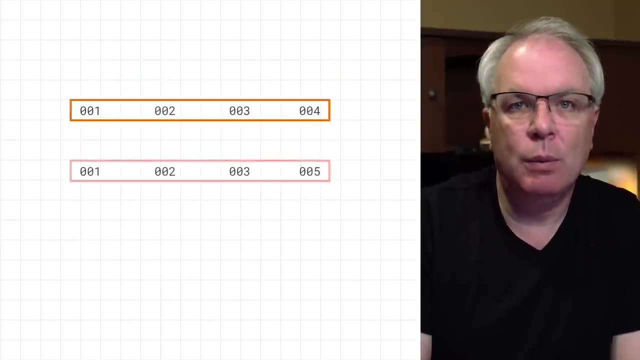 so I can just use one, two and three again for them, And I can create a new number for cat, which I'll say is number five. So now my sentences are one, two, three, four and one, two, three. 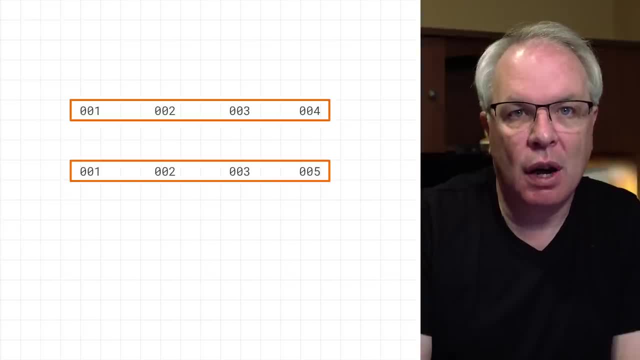 five. What's interesting here is, now that the words are gone and the tokens for the words are just used, we can begin to tell that there's a similarity between the sentences, So maybe we're beginning to get a glimpse at what it might look like. 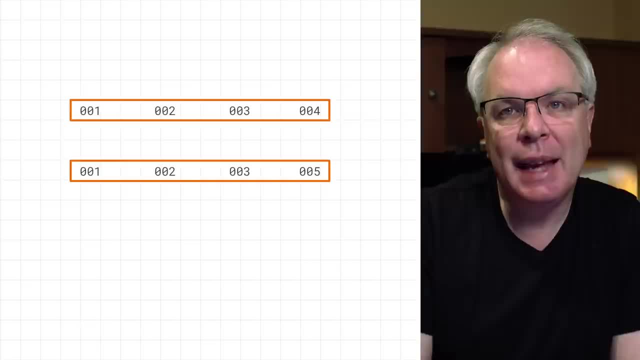 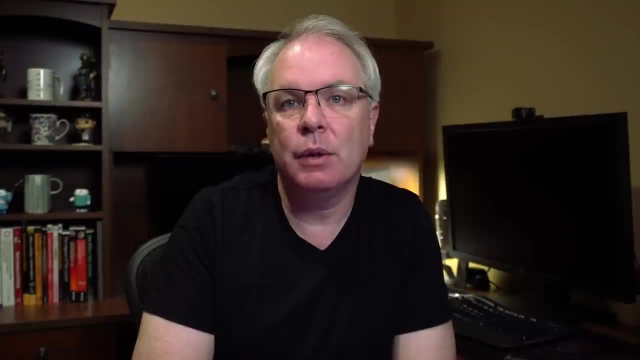 To have sentences turned into numbers yet maintain some kind of meaning. The process I just outlined is called tokenization, and it's an inherent part of doing natural language processing, or NLP. TensorFlow gives you APIs that help you to achieve this very simply. 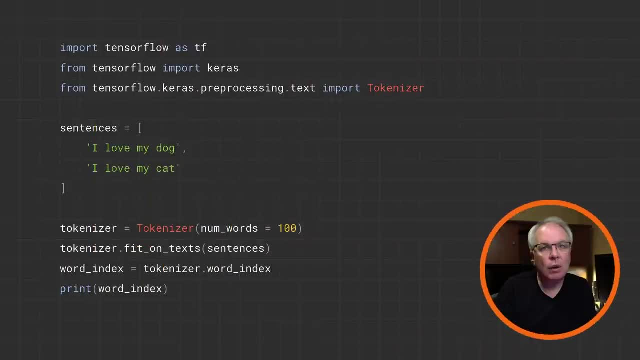 We'll take a look at them next. Here's all the code that you would need to tokenize the sentences I showed earlier. We can break it down and go through it line by line. The tokenizer tool, for example, is part of the TensorFlow Keras libraries and they're in the preprocessing. 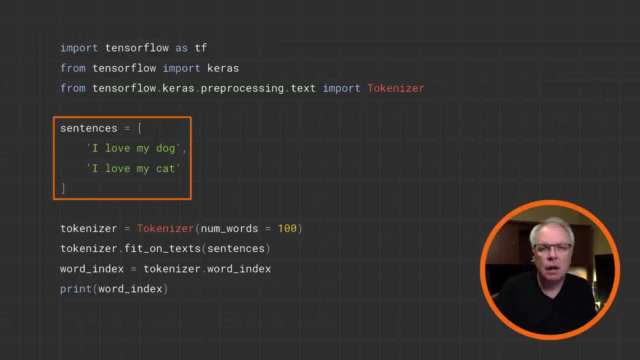 namespace, So make sure you import these. I'm going to hard code the sentences into an array Now, while this is a super simple corpus- there's just two sentences and five unique words- this design pattern can work for much bigger sets of data. You'll soon be working with tens. 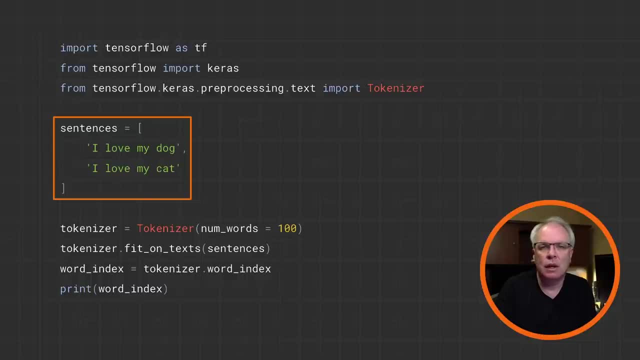 of thousands of sentences with thousands of unique words, and it's all pretty much the same code. So don't worry right now if this looks a little bit too simplistic. You can then create a tokenizer with a lowercase t by simply creating an instance of the tokenizer. 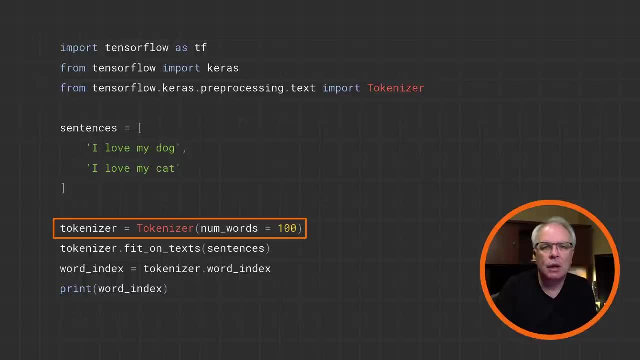 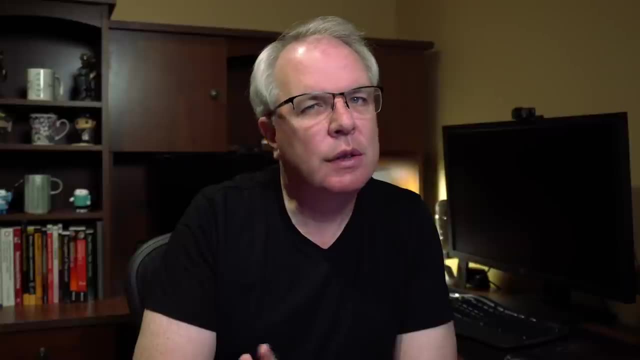 uppercase T and initializing that with parameters. One of these is the numWords parameter, which specifies the maximum number of words that you want to care about. There's only five unique words here, so it doesn't really make a difference, but with larger sets of text it can. You'll. 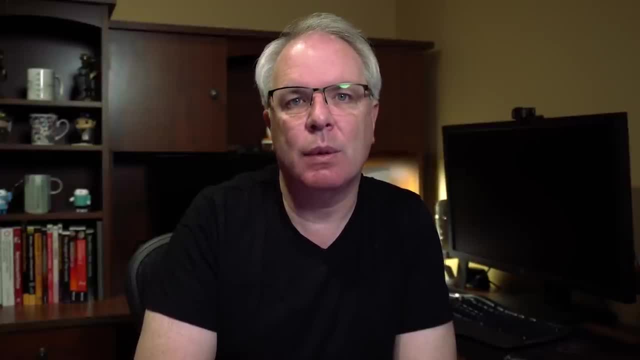 commonly encounter bodies of text with many thousands of unique words in them, and lots of these words may be unique in their own way. So you can create a tokenizer with a lowercase t, and the number of these words may be only used once or twice By specifying the number of words. 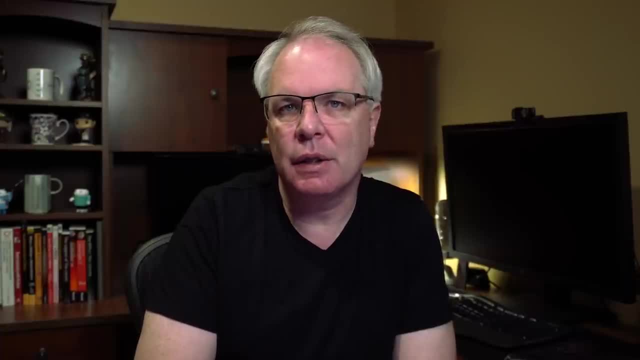 that you care about in your tokenizer, you get an easy way to filter those out. The tokenizer is smart enough to assign tokens to words based on how commonly used they are in the corpus. So the most common word will be at index one, the next common word will be index two, etc. 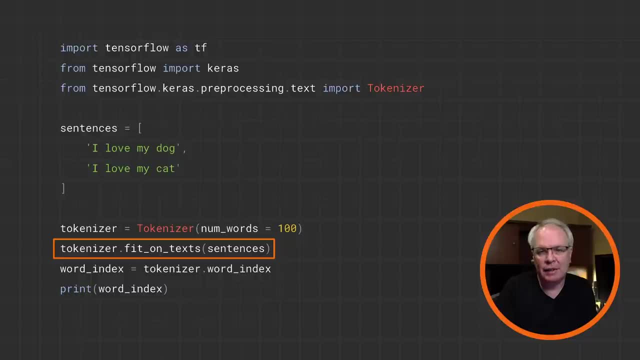 To get the tokenizer to do its job, you can fit it on texts and pass it your corpus of text. In this case it's our simple array of sentences To see the word index that the tokenizer created. you can just get the word index property. 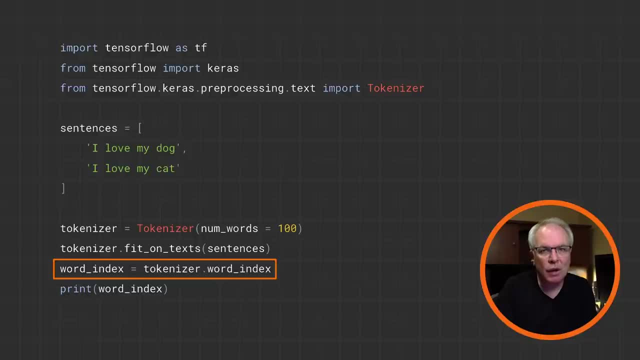 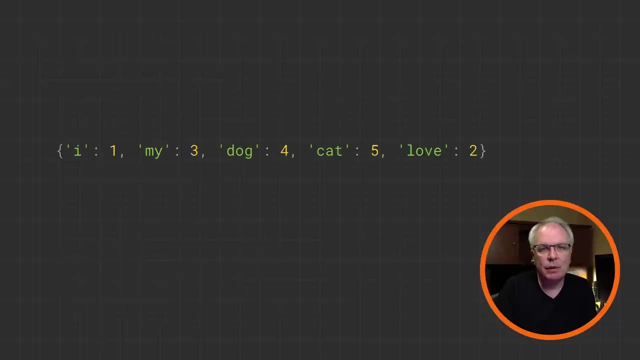 This will give you a set of name-value pairs where the name is the word and the value is the token for that word, And then you can just print this to inspect it. When you print it out, it won't necessarily be in any order, but keep an eye on the values. 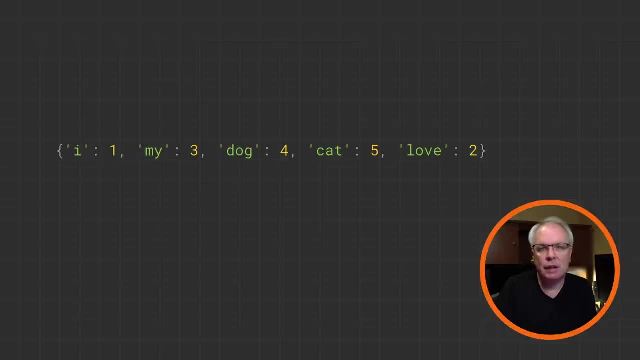 Like I said earlier, the most common words will be the lowest index And in this set I love my appears twice, while dog and cat both appear once. So I love my are the lower indexed words, one, two and three, and dog and cat are the higher indexed ones: four and five. 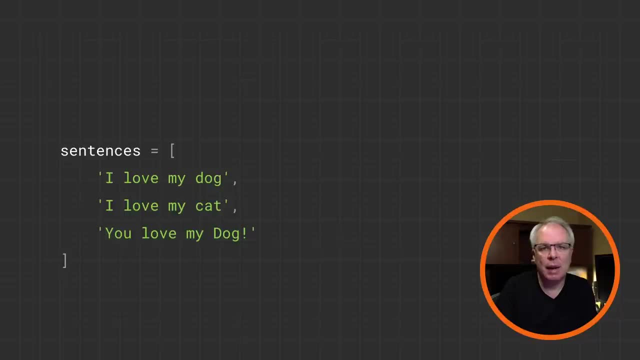 So what if we expand our sentences and then add some more content, like maybe you love my dog, with an exclamation mark- And note that exclamation. The default behavior of the tokenizer is to strip punctuation out. like this It can be overridden. 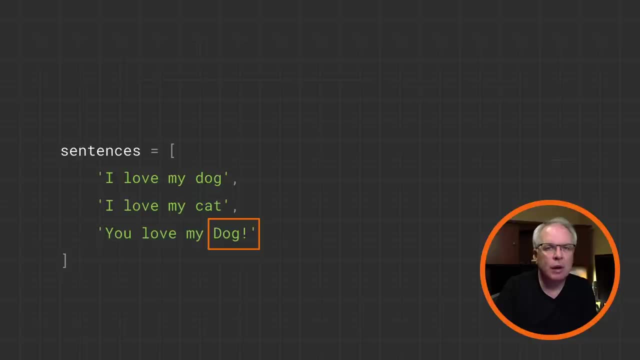 but we'll keep it in for now. It also makes all of the words become lowercase, so my capital D dog will be treated in the same way as a lowercase d dog. The tokens will now look like this. Notice that they've moved around. 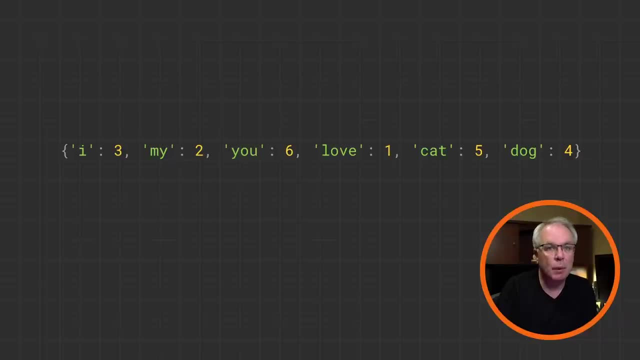 a little Love is now the number one token because it's the most used word and it's similar with my. Also notice that dog lost its exclamation and there's only one token in here for dog and it represents both usages of the word, despite the exclamation being on the second one. 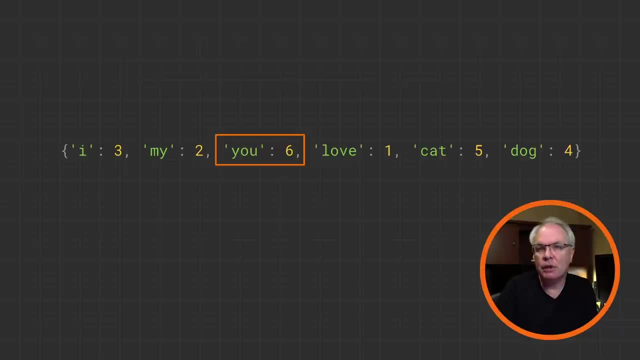 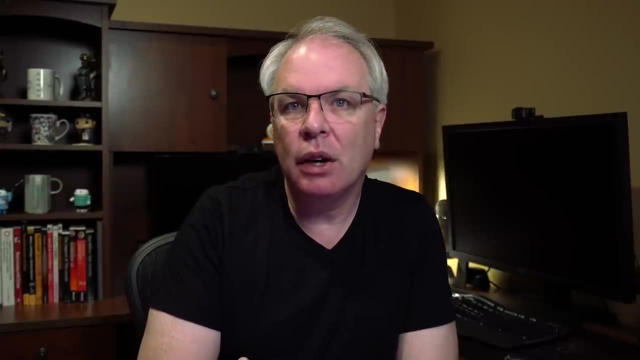 We've added a new word, you, because that was first used in the new sentence that was added to the corpus, So I hope you found that pretty straightforward, despite the underlying power in the tokenizer. Next up, I'm going to step through a collab with the code for all of this. 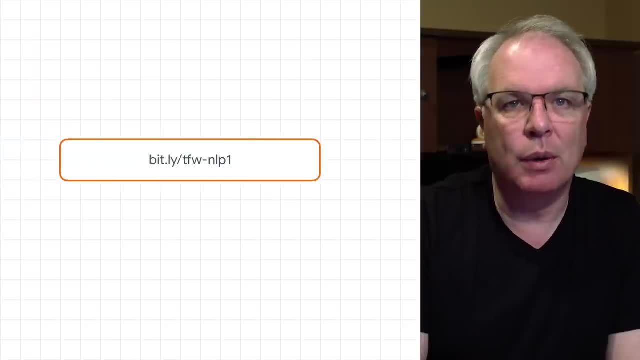 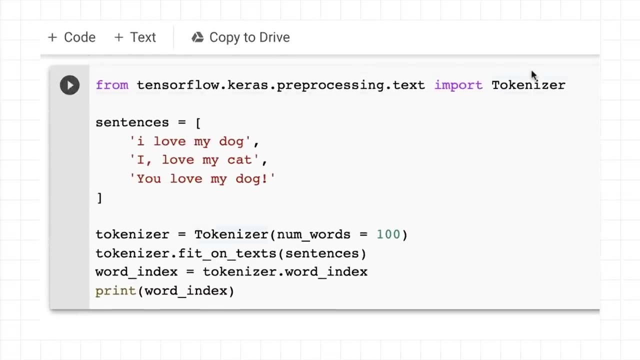 and then you can try it out for yourself. Okay, here's the URL of that collab. Pause the video to give it a try for yourself. This is the code that we were looking at in the videos. Here we can see we're going to import the tokenizer and I have an. 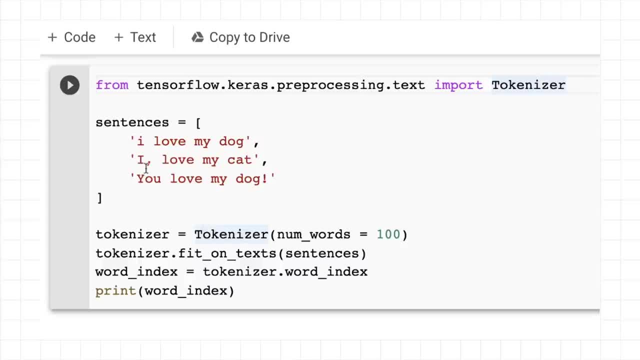 index and we're going to add a number of sentences here: I love my dog, lowercase I. I comma: love my cat- uppercase I, and things like you love my dog, with an exclamation. We'll then use the tokenizer and we'll fit it on the text of these sentences. 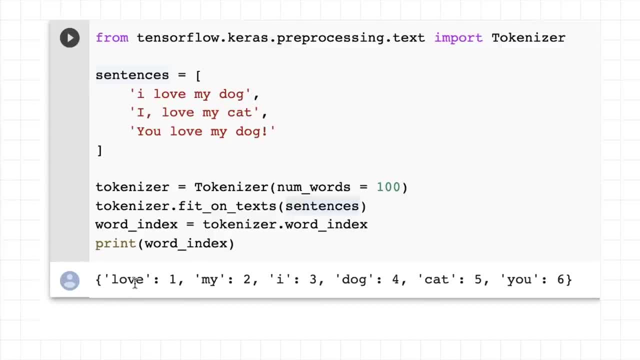 and take a look at the word index. So here, if we take a look at the word index, we'll see that the word love is indexed as number one. It became token number one and that's because love was used the most. It was also my was used the most as well, There. 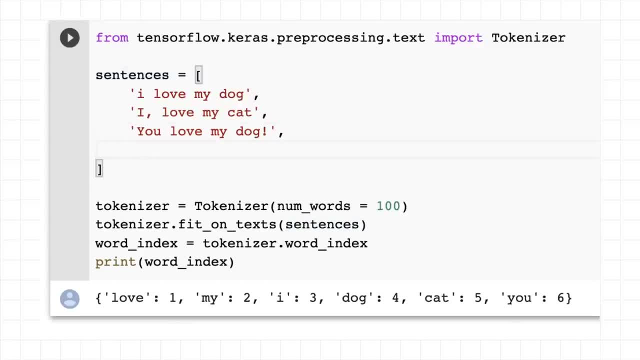 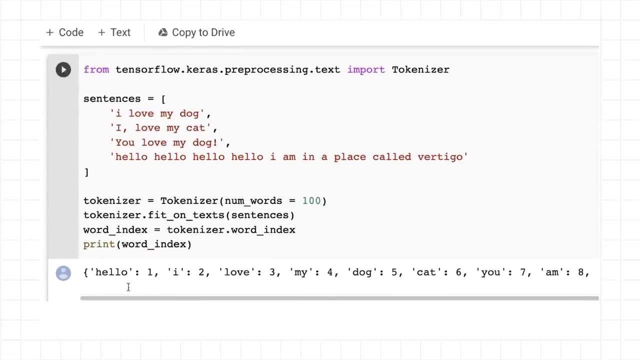 are three of those, just like love, and you can see they're at the top of the index. For example, if I were to add another sentence here like hello, hello, hello, hello. I am in a place called Vertigo, and then I were to run it on this, then we'd see hello is now. 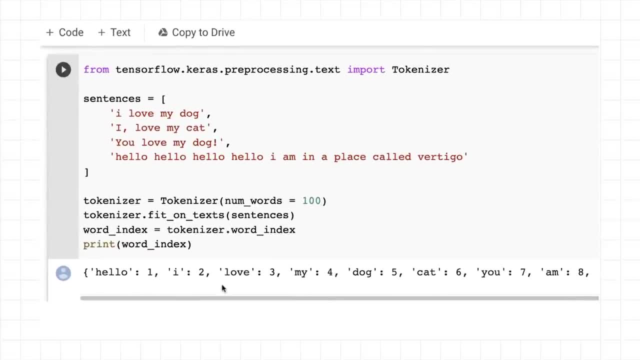 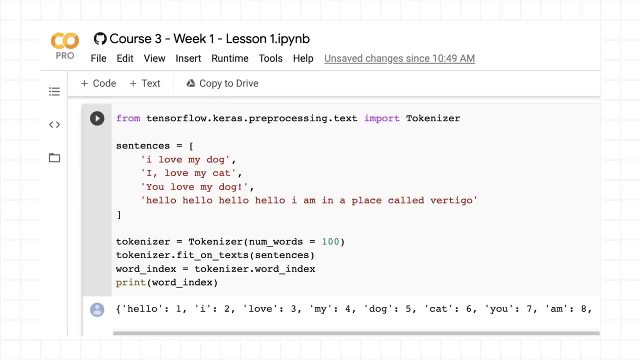 the top one because there are four of them, where there are three loves and three mys, that kind of thing. Oh, I also now shows up because there are three I's. This is basically how the tokenizer works. Hopefully this will be useful for you. 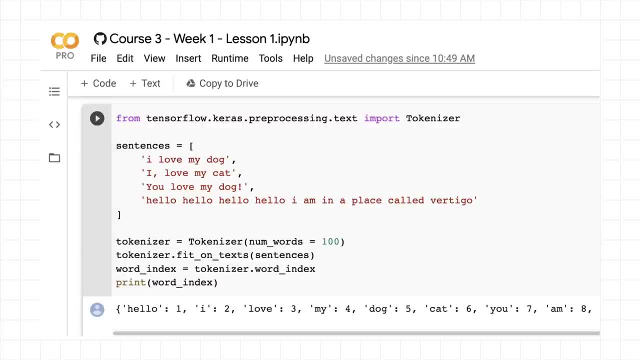 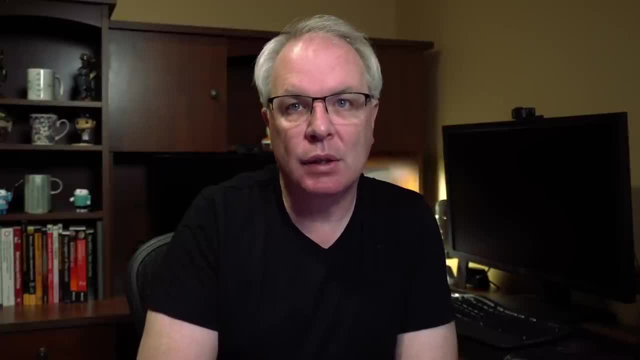 Have a play with this code. Try some examples yourself and see what you can come up with Great. I hope that was easy for you. In this video, you got your first taste of NLP using tokenization, where you were able to take sentences and have their words encoded into tokens. 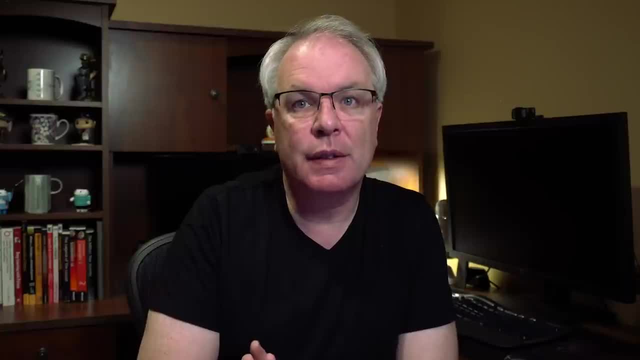 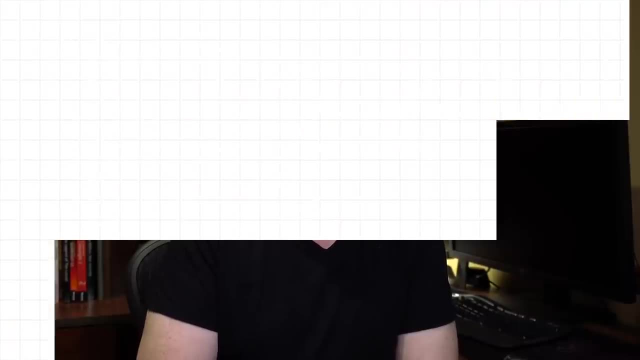 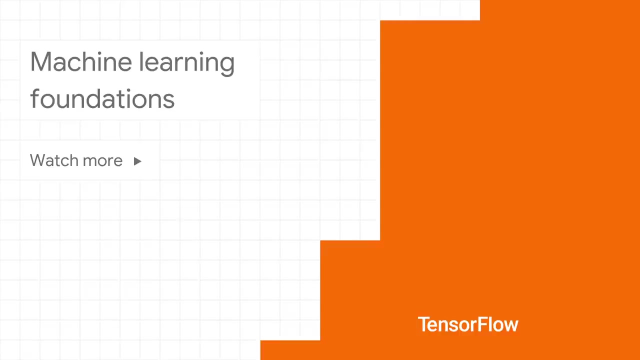 The next step on your journey is to replace your sentences with sequences of tokens. You'll see that in the next video, so don't forget to hit that subscribe button and I'll see you there. Bye-bye.